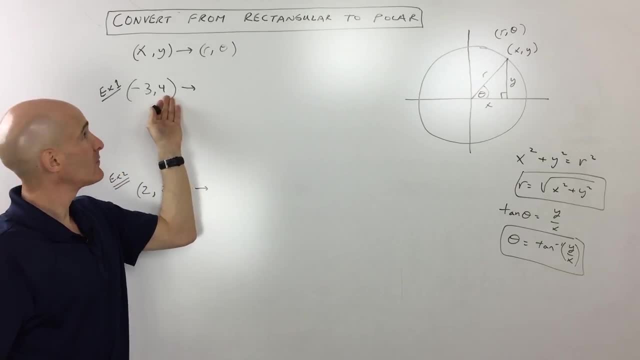 Let's look at example number one. to give us the point negative 3, 4.. That's XY rectangular coordinates. We want to get to R theta, So I always like to draw a sketch. I just kind of like to see what's going on here. 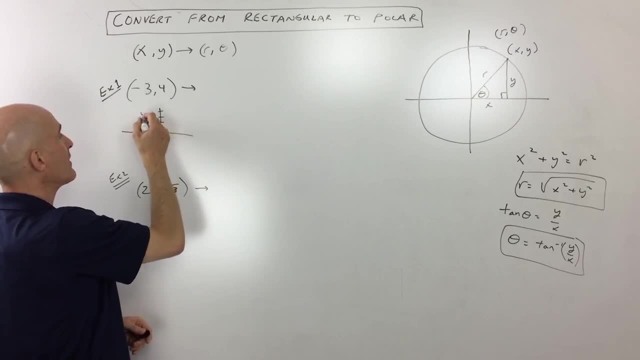 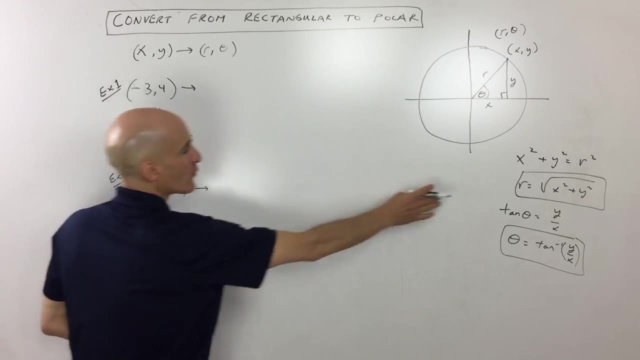 So left 3, up 4.. That's the point. That's the radius we're looking for. That's the angle. That's the angle we're looking for. Okay, so you're with me so far. So what we're going to do is we're going to use this first formula over here. 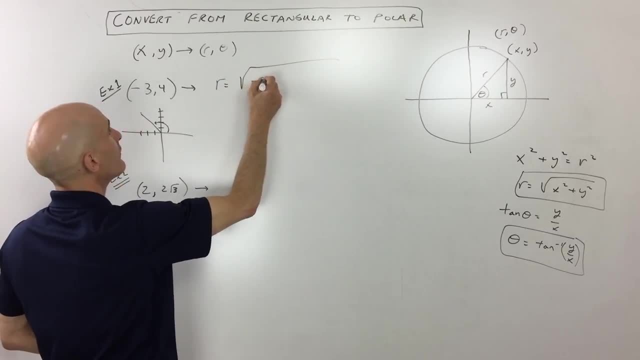 We've got. the radius is equal to the square root of X squared, So negative 3 squared plus Y squared, That's 4 squared. So this comes out to 9 plus 16. squared of 25 is equal to 5.. 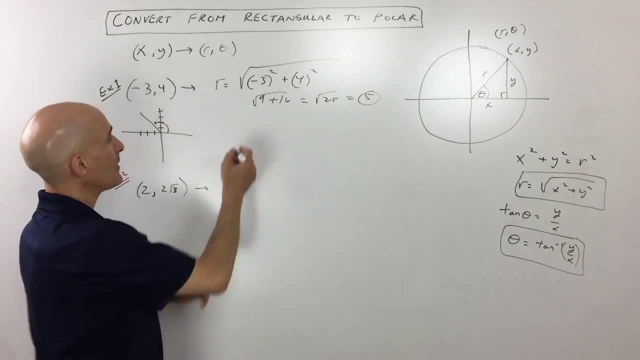 So we know our radius is 5.. Okay, now we want to find the angle. So we're going to be using this formula over here: Theta is equal to the tangent inverse of Y: Y over X. Okay, in this case Y is 4 and X is negative 3.. 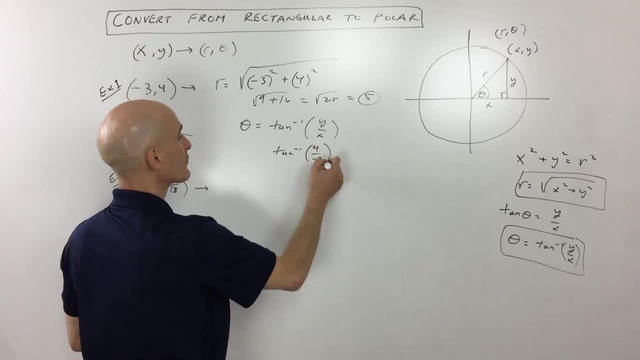 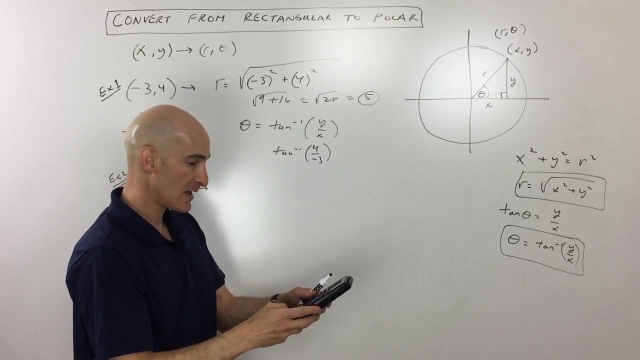 So we're doing the tangent inverse of 4 over negative 3.. Now let me go to the calculator on this one. See what that comes out to. We've got tangent inverse of 4 divided by negative 3. And that's coming out to negative 53.1.. 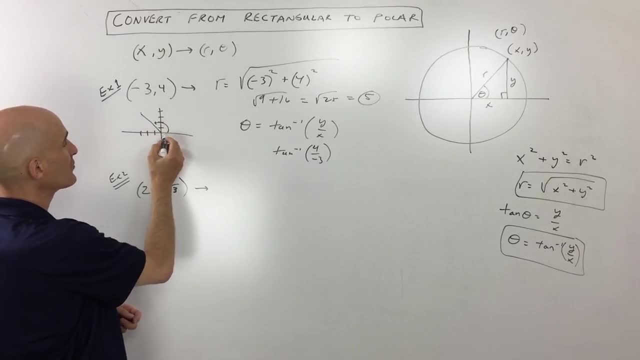 But you're probably saying: wait a second, Mario, That's actually not a negative 53.1.. This is a negative 53.1 here. So what you do in that case is because we're over here in the second quadrant. 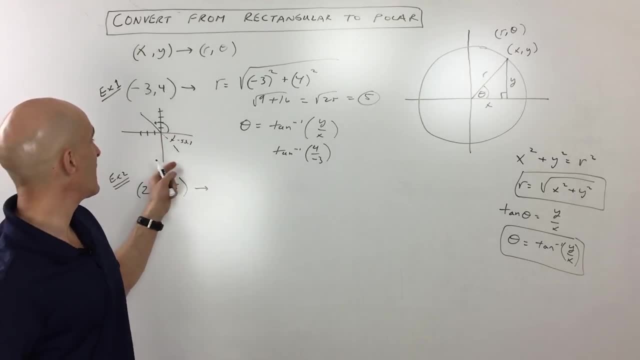 you have to add 100. So we're going to add 180 degrees. Tangent is restricted from negative 90 to positive 90. That's why it's giving me this answer. So if we add 180, we're getting about. I'm going to round to about 127 degrees. 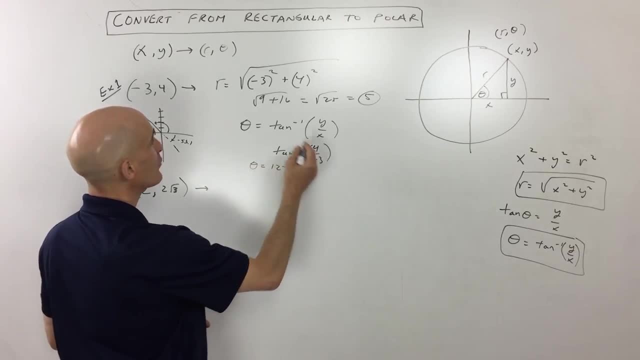 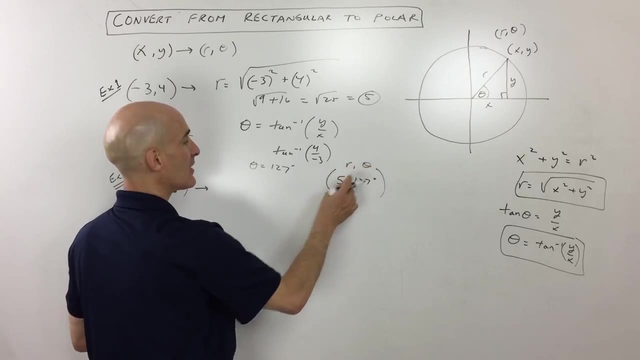 Okay, so that's our angle. Theta equals 127 degrees. If we put it together, the radius and the angle, 5, 127 degrees. That's our theta and that's our point in polar coordinates. Okay, so now, for example, number 2, they're giving us X and Y, right. 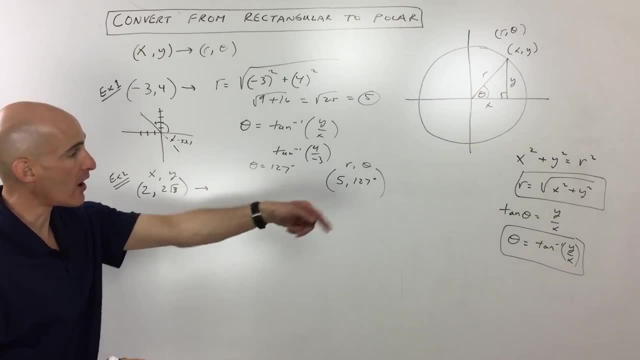 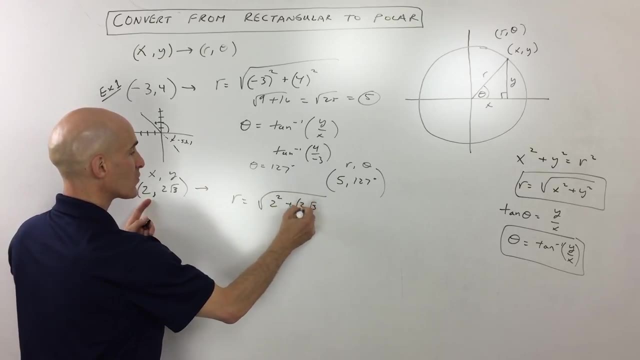 So 2 and 2 root 3.. And we want to go to polar R and theta. So let's use this formula: R is equal to square root of X squared plus Y squared. Take the square root So that comes out to 4 plus, let's see, 2 squared is 4..